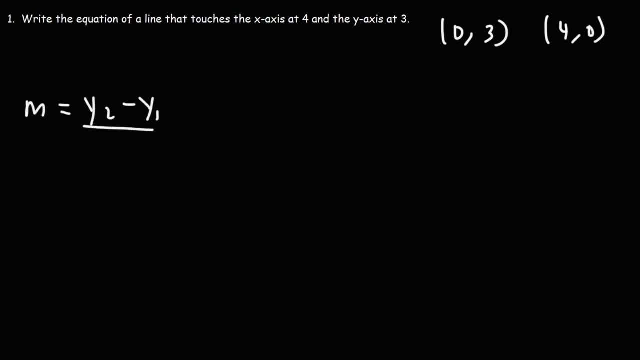 So m is equal to y2 minus y1 over x2 minus x1. Let's call this x1,. therefore, this will be y1. This will be x2, and the other one will be y2.. If you switch x1, y1 with x2 and y2, you will still get the same answer. 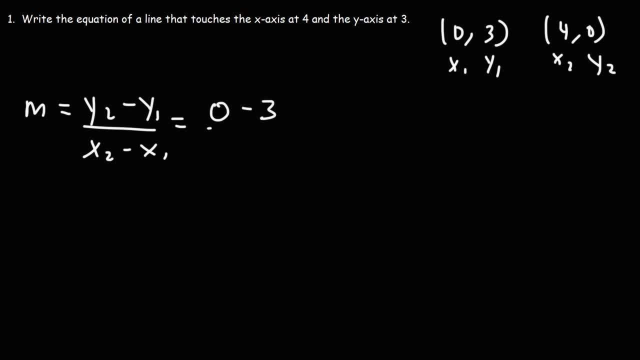 So y2 is 0, y1 is 3, x2 is 4, x1 is 0. So this is negative, Negative 3 over 4.. So now that we know the slope and we also know the y-intercept, 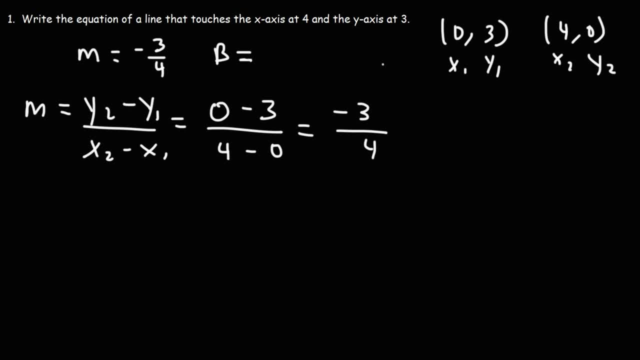 the y-intercept, which is b. that is this value here, That's 3.. We can now write the equation of the line in slope-intercept form. So using the formula, y is equal to mx plus b. it's going to be: y is equal to negative 3 over 4 times x plus 3.. 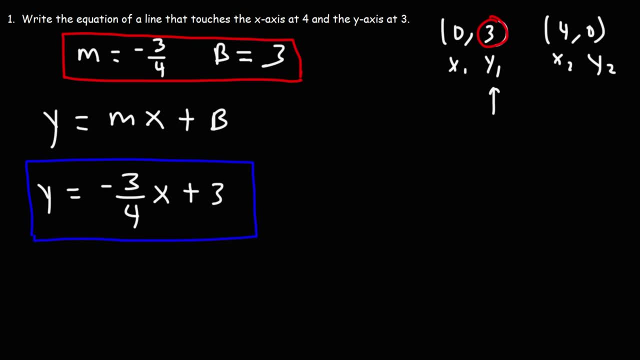 So that's the answer in slope-intercept form. You can also convert it to other formats, like standard form and point-slope form, but we're not going to focus on that in this video. Now let's try another similar problem. Let's write the equation of a line. 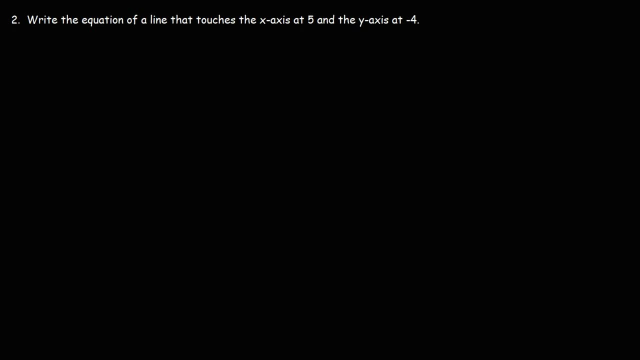 Where this line has an x-intercept of 5 and a y-intercept of negative 4.. If you want to pause the video to work on it, feel free to do so. So let's convert it to ordered pairs. Let's start with the x-intercept. 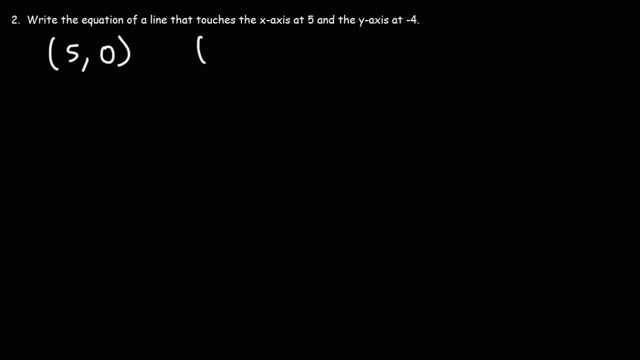 It has an x-value of 5, a y-value of 0.. The y-intercept has an x-value of 0, but a y-value of negative 4.. We're going to call this x1, y1, and this one's going to be x2, y2.. 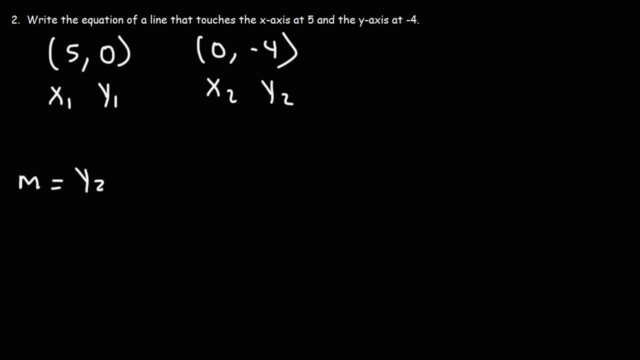 so now that we have the two points, let's calculate the slope of the line that passes through those two points. so y2 is negative 4 minus y1, which is 0. divided by x2 minus x1, which is 5, so this is negative 4 over negative 5. the two negatives will cancel, so we get positive 4 over.